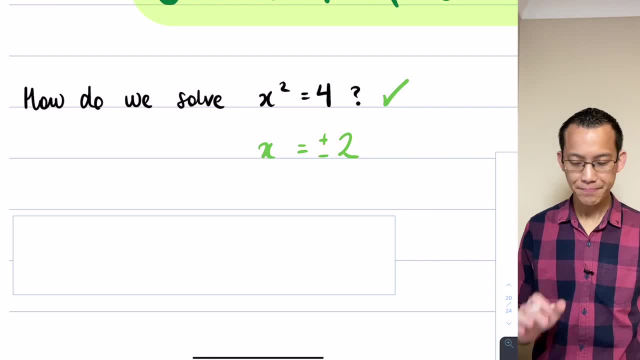 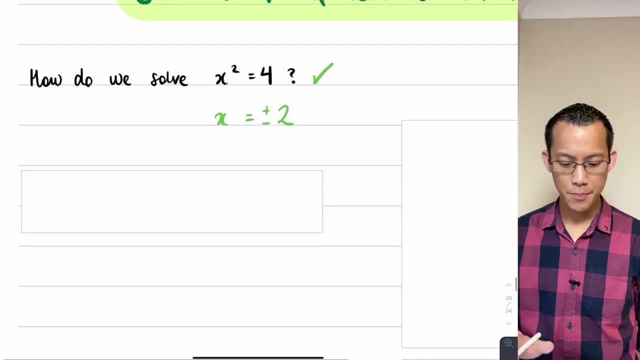 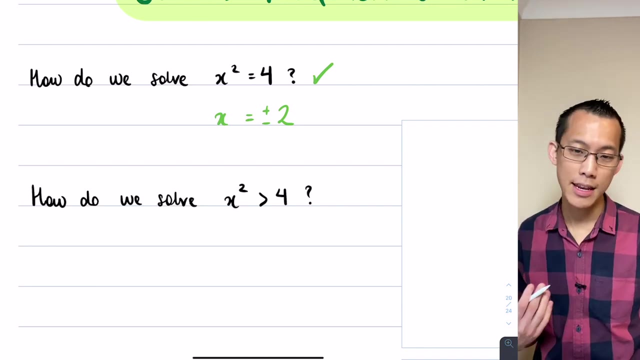 four, so they both satisfy the original equation. Okay, so we know how to solve equations- no big deal. but I want to highlight for you that, even though in many ways they're similar, inequalities like this are different in some really crucial ways, which make the graphing techniques that 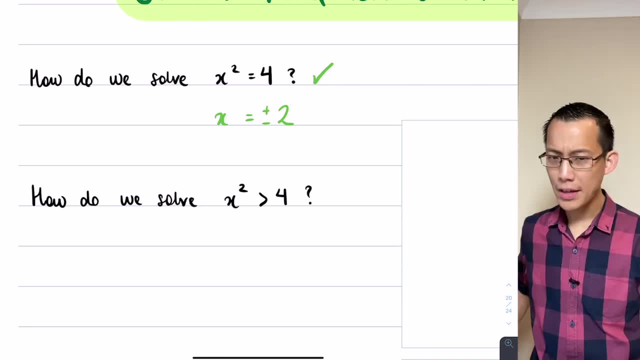 we've been looking at recently, very, very relevant and useful. Let's just imagine for a second- please don't write this down because I'm about to run out of time. Write down something wrong. This time I'm doing it on purpose. Imagine if we were to try and. 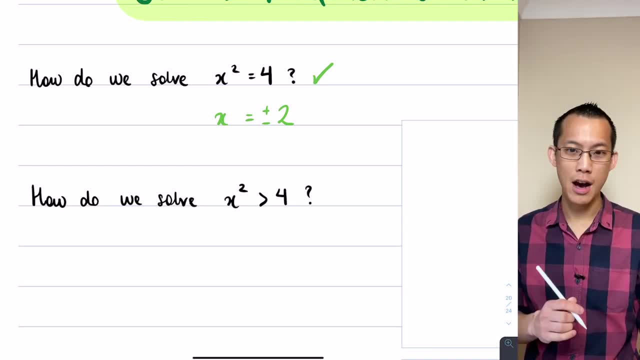 treat this inequality the way we treated the equation up above. If I were to say, okay, well, I've got an x squared, but I just want x, So I'll do the same thing, I'll take square roots of both sides. That leaves me with x. on the left-hand side There's a greater than symbol instead of. 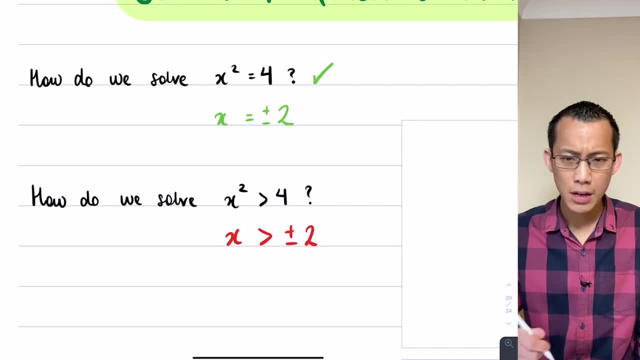 an equal sign. And then I say I get plus or minus two on the right-hand side. Now this is weird because it's not just a square root, it's a plus or minus two on the right-hand side. It's also wrong. And it's weird firstly because we know that this guy up here is shorthand. 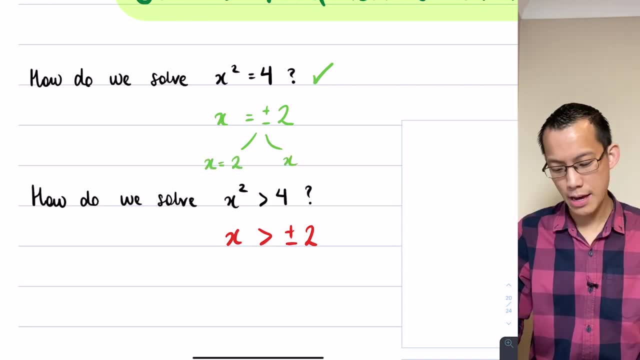 It's short for x equals positive two and also x equals negative two. It's shorthand for both of those at the same time. But when you have a look at this guy, I've written in red which is wrong. if you imagine splitting it off in the same way, it would be kind of puzzling. You would say: 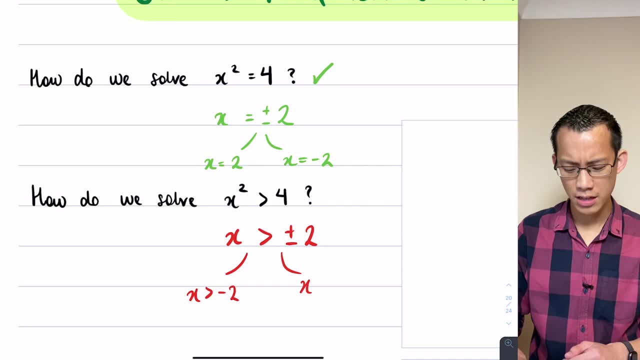 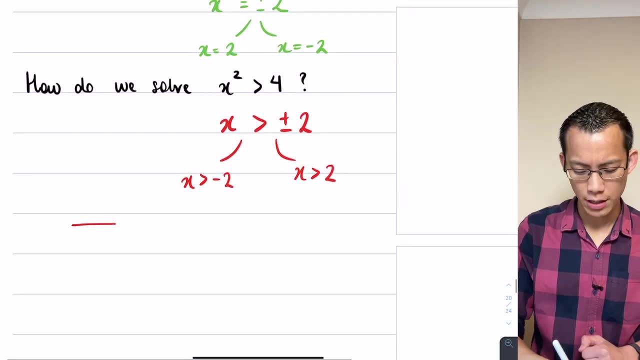 well, x is greater than negative two. And then x is also greater than two. Now that's kind of weird, right, Like if I were to draw a square root I would say, well, x is greater than negative two. And if I were to draw this on a number line, for example, if I drew and I invite. 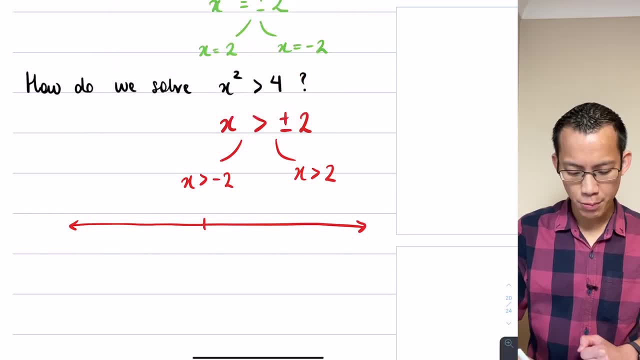 you to have a think about what this would look like for you if I put some markings here, that'll do me. And I said, okay, let's plop zero there in the middle of the number line. Here's two, here's negative two. What would I, or how would I, represent these two inequalities? 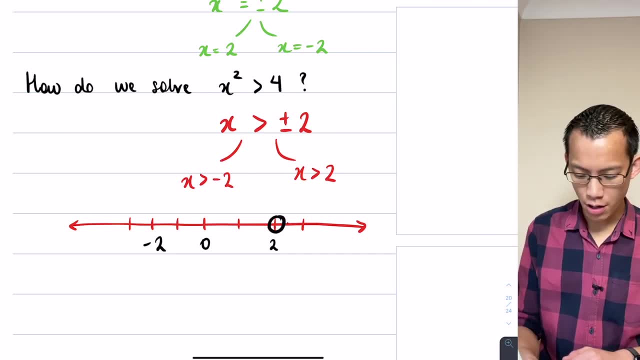 on the number line. Well, x is greater than two, will be this guy over here on the right-hand side from two onwards. And then when I look at the other one, x is greater than negative two. I draw another hollow circle And then I sort of just keep going right And it sort of includes: 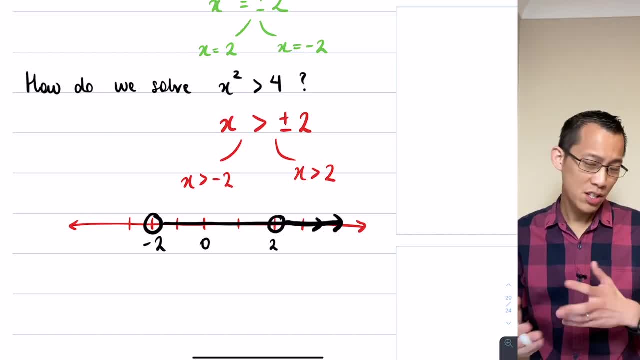 the other one. Now, not only is this confusing, it's just plain wrong. If you take some values that are actually in this part of the region that I've drawn, let's take a value like here: one right When I put in x equals one, does that solve this inequality up here? And the answer is: 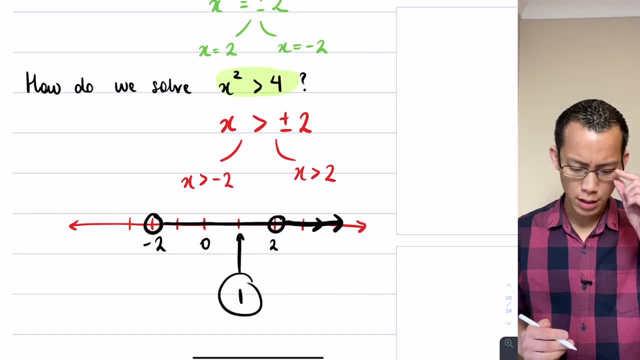 it definitely does not. You substitute in: x equals one. you're like one squared That's not greater than four. Okay, So I'm going to take a value that's greater than four, And I'm going to take a value that's greater than four, And I'm going to take a value that's greater than four And I'm 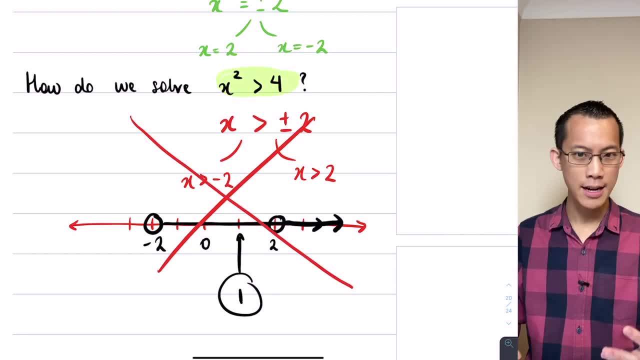 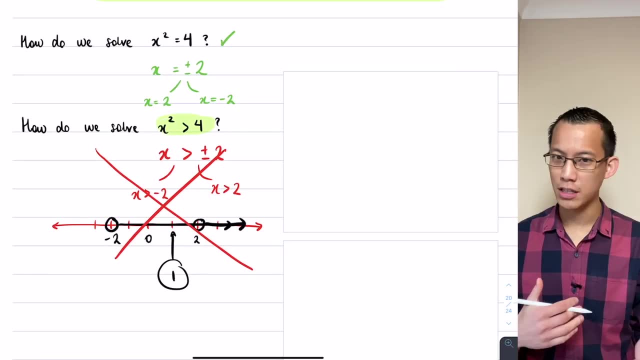 This is not satisfactory. We can't just treat an inequality the way we treat an equation. There are some parallels, like we can add and subtract the same thing to both sides. We can multiply by a positive number on both sides and everything will be fine. But when it comes to 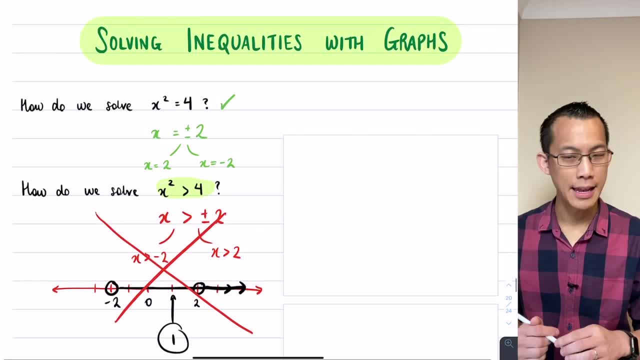 solving things like this, we have to try a different technique, And that's where the heading, this idea, comes into mind. We're going to use graphs to help us This time. please do pick up pens and write and draw along with me. I want us to take this inequality: this x squared is greater. 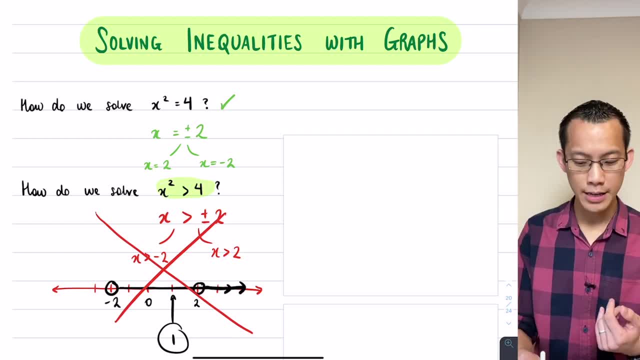 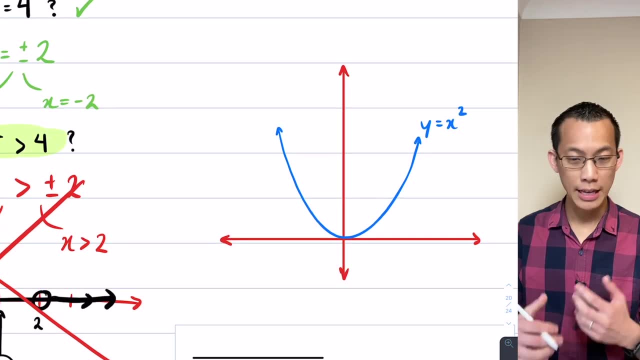 than four, and I want us to visualize it with the help of all the graphing techniques we've developed over the last couple of weeks. This is what x squared looks like. We know that right y equals x. squared gives us this parabola shape. Now, when we see this inequality over here, 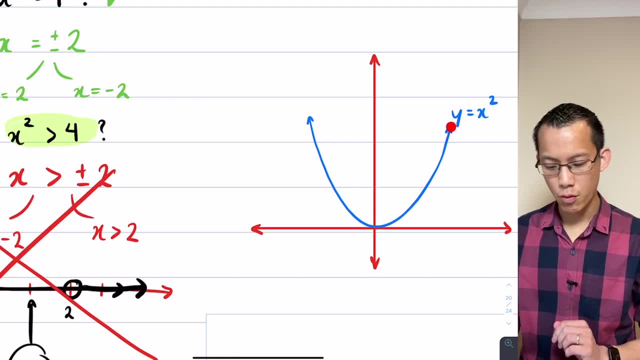 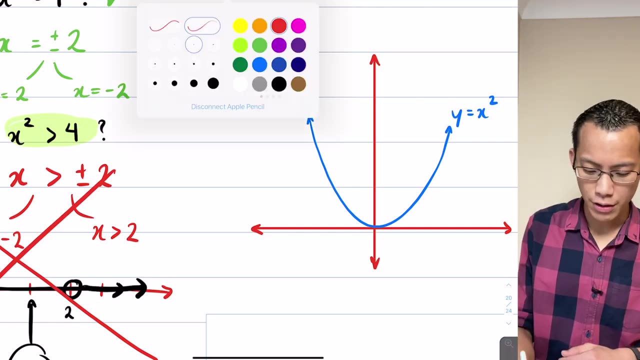 what this is asking is, when you look at this graph x squared, can you tell me when is this graph above four? I should say, when is it above y equals four? Okay, Y equals four is a horizontal line. I'm just going to draw it in now. Let's say it's somewhere around there. Here's: y equals four. 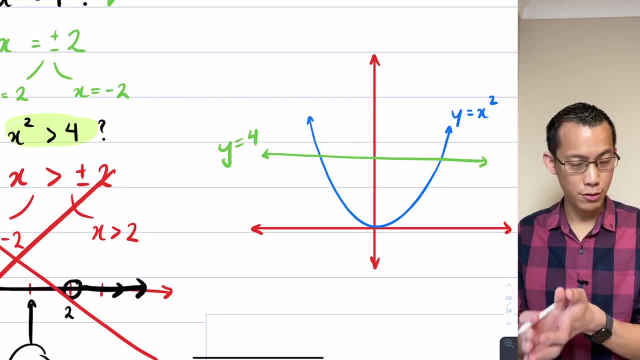 And you can clearly see that there are two parts of this graph, two parts of the parabola that are above my green line right, And those are the parts that I'm interested in. You can see, there's this section up here. I'm going to make this. 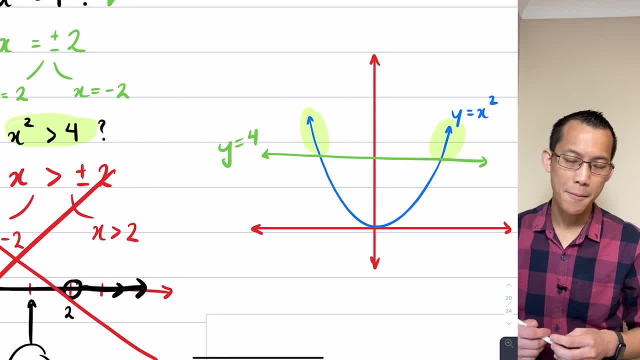 a bit thicker, and then you've also got this section over here. both of these sections of the graph satisfy this. this quality I'm looking for. when is x squared? when is the parabola above this line 4? and now, what I want to do, though, is I: 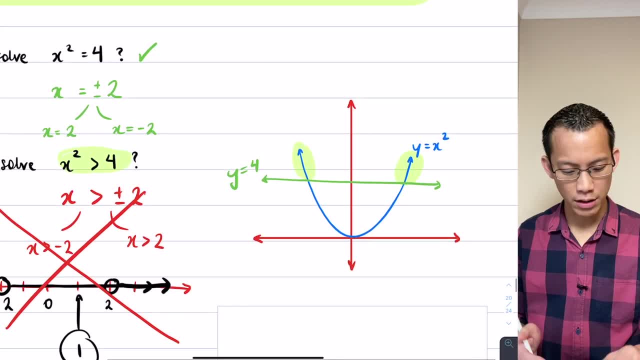 want to say: what are the x values that make sense of that? like, when you had a look at me solving this equation over here, I got x values that were the solution. what are the x values that make sense of this? well, what I do is I look. 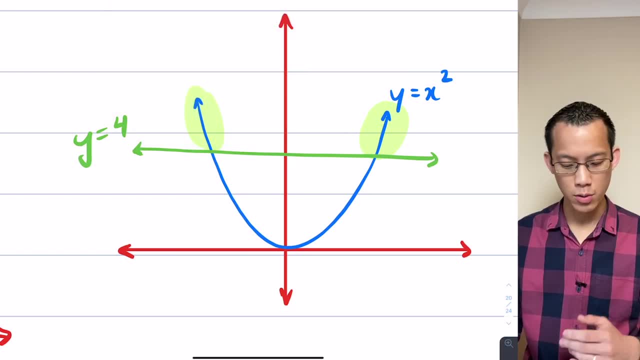 at the portions of the graph that are satisfying this quality. it's. it's this part over here on the left and this part over here on the right, and I look for the domain of the function that gives me those parts of the graph. okay, let me say: 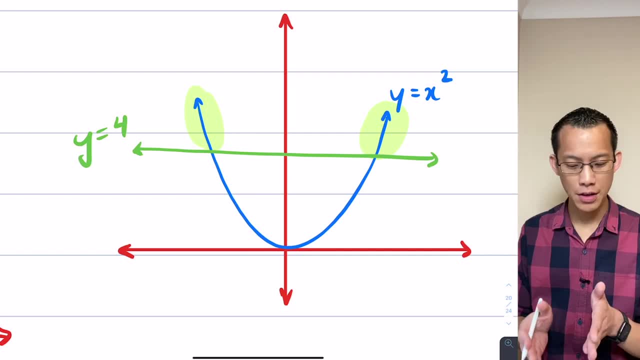 that one more time I'm looking for the domain of the function that gives me the parts of the graph that I want. so, for example, if you have a look downward here, if I go from this spot over here and to the left, you can see that all the parts. 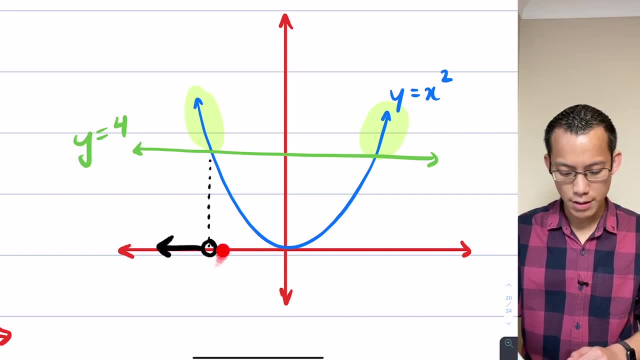 of the parabola that are two-dimensional, are actually two-dimensional, and that's to the left of this little coordinate. here. all the parts to the left will be up above y equals 4, so I want those sections right. all I need to know is: what is this spot? where is this point of collision? now, based on what we did with 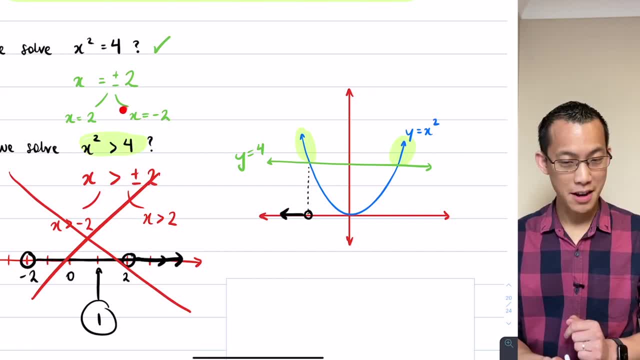 this earlier question over here you can see that's going to be. x equals negative 2. that's going to be the value that comes down here. so so long as I am to the left of negative 2, I guess we would say x is less than. 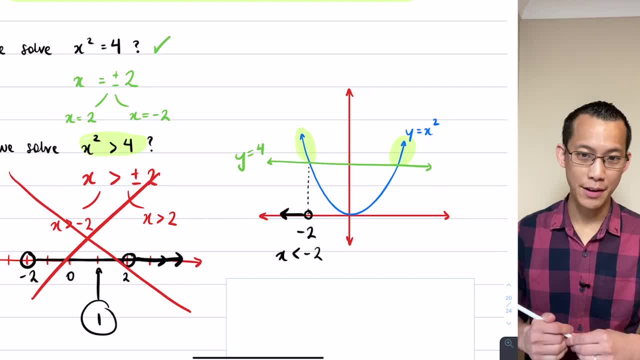 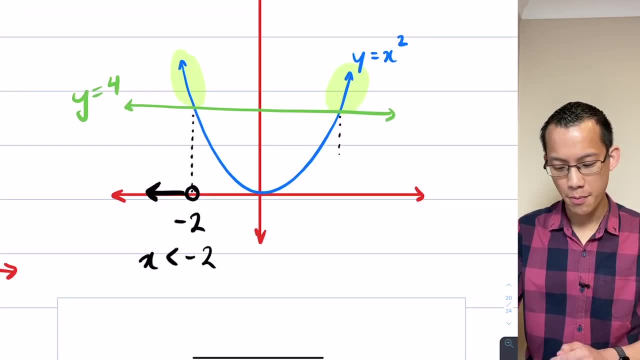 negative 2, that part will be above. y equals 4 and it's the part that I want. then, of course, if you look over to the right, there's this other section over here that comes from this spot going in the positive direction. so so long as I'm to the right, 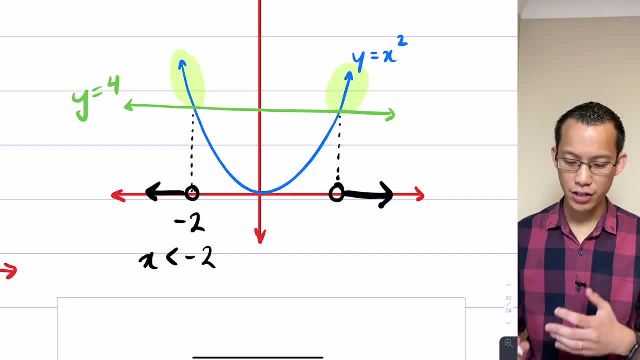 of that if I'm in that domain. again, that section of the parabola which you can see up above here, it's above: y equals 4 and that's the part that I'm interested in. so again, I need to know what this value is. it's 2, based on that question, I. 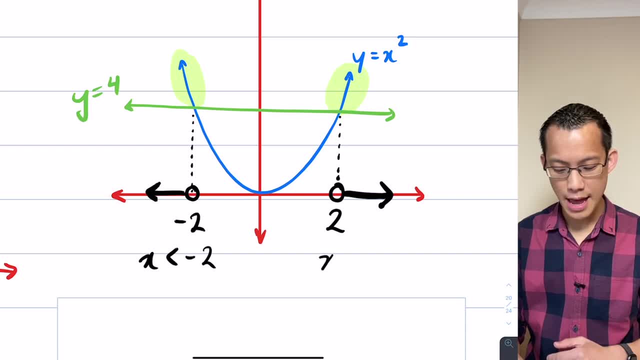 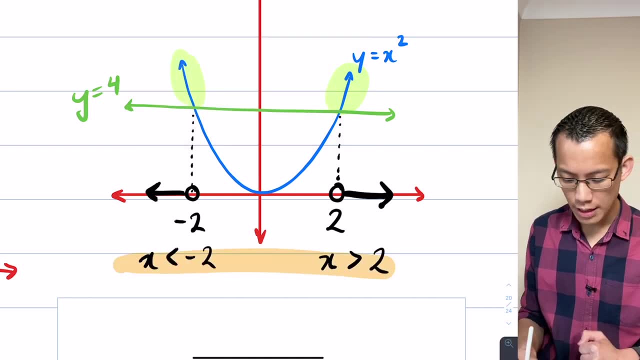 solved before and I want the part to the right of it. so it would be: x is greater than 2. now, what I've written in here- let me just highlight this in another color for you- what I've written in here is my actual answer. it's: x is less than negative 2, or? 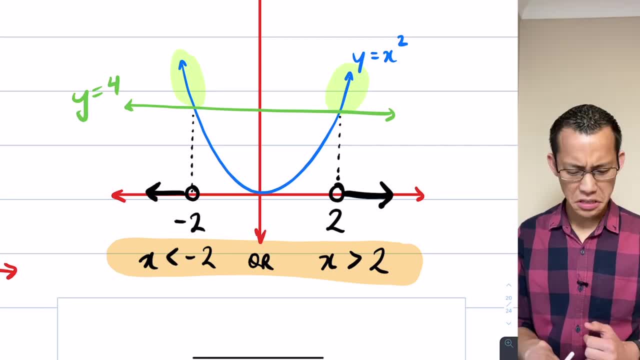 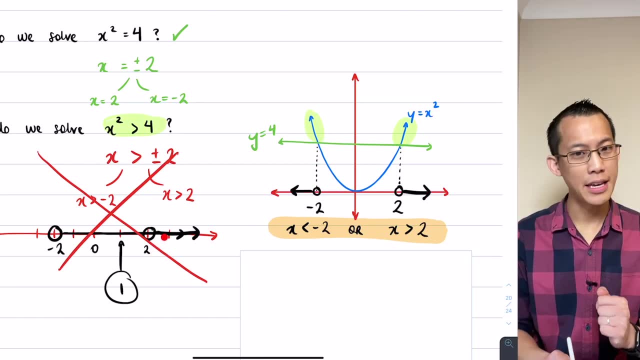 x is greater than positive 2. so you can see it's it's kind of related to what I did over here, which was incorrect, but the inequalities are facing in different directions and I can tell that because I'm looking at a graph. the graph, rather than algebra, is going to be our key instrument for solving. 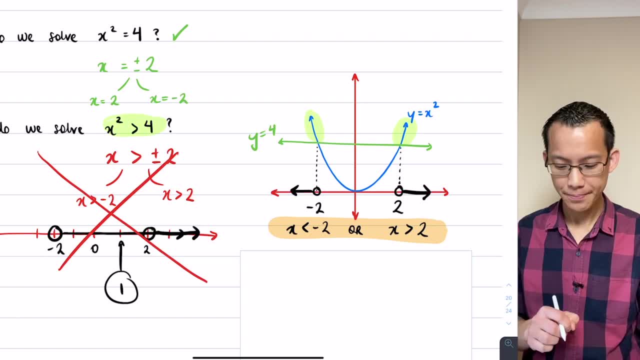 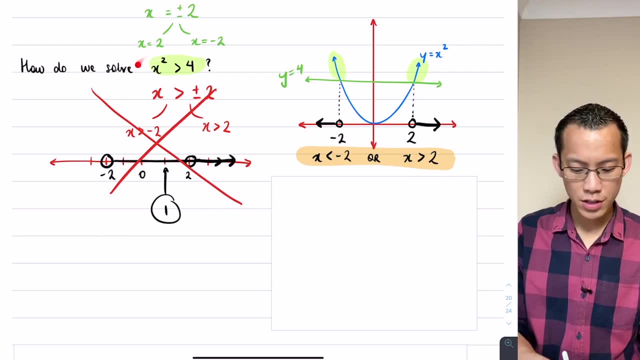 questions like this for solving inequalities. now, just before I pause and see if mrs Lee's has anything to add, I want you to notice that this is not the only way we can think about this. x squared is greater than 4. I could take this original question- let's go down here- and I could rearrange it slightly. I. 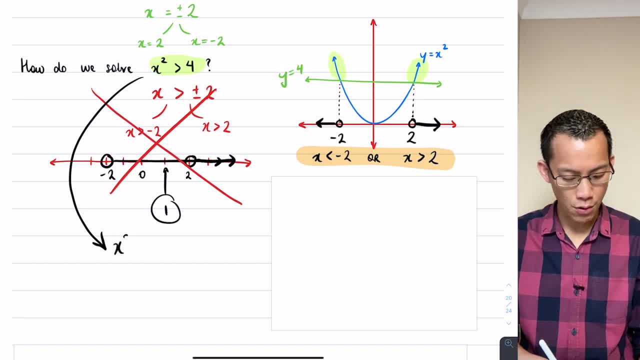 could say: well, what about if I subtract 4 from both sides, I would get this right now. the reason why I'm highlighting to do this is because what I'm now looking at is a single function over here on the left, and what I want to know is: when is 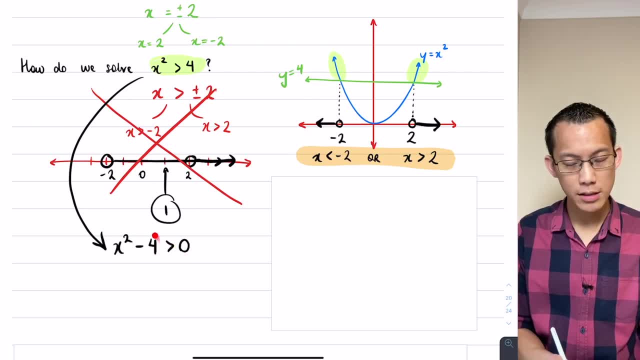 that greater than 0. in other words, when is this function on the left? when is it positive? now, the reason I like that is because it's really easy to spot where functions are positive and where they're negative. we've got a place on our Cartesian plane that sort of divides the positive from the negative, and that is. 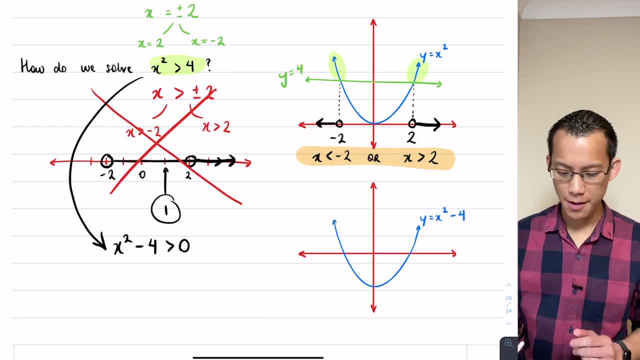 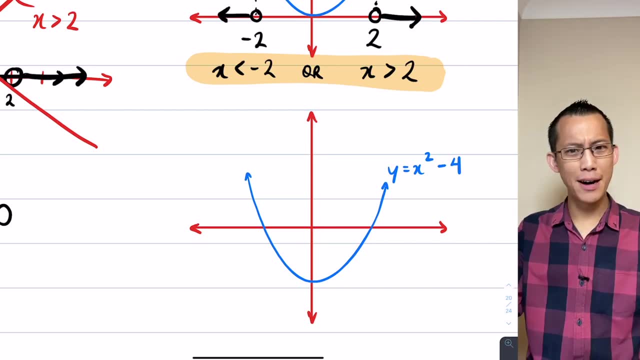 the x-axis. if you have a look at this guy over here, you can see this is the same graph. it's being translated downwards four units and what I'm now looking for is where's the part that's above the x-axis. I don't have to draw some other line here in green, I just look at the axis which I 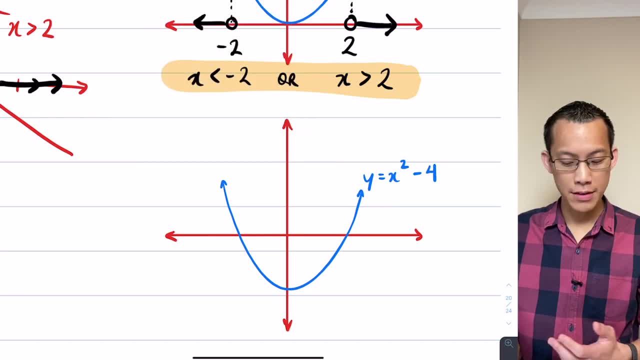 had to draw anyway and I say: where is the part that is above the axis? you can see, it's the same part over here on the left and this same part here over on the right, and if you go ahead and you solve this, you're going to get this same. 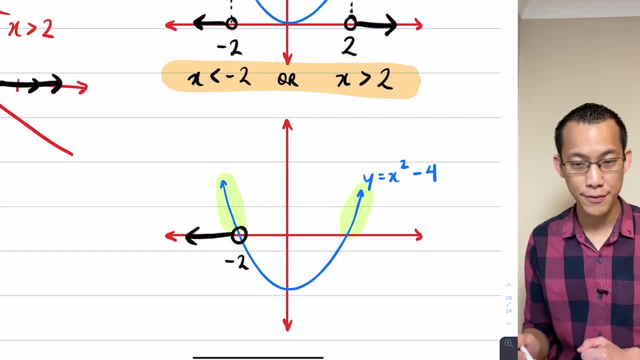 intercept over here: negative 2, and it's the section to the left of that, and then you're going to get the on the right, which is positive 2, and you're going to go in the positive direction. so you can see, you get the same answer. but I like thinking about it. 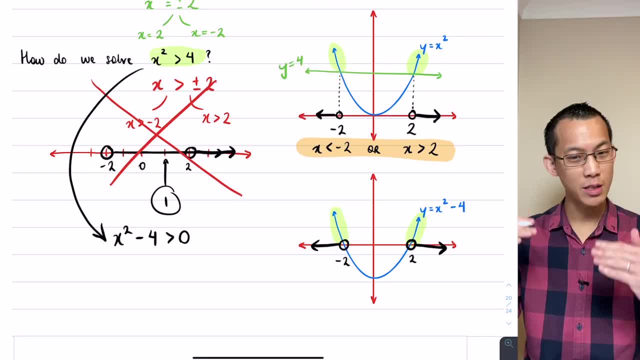 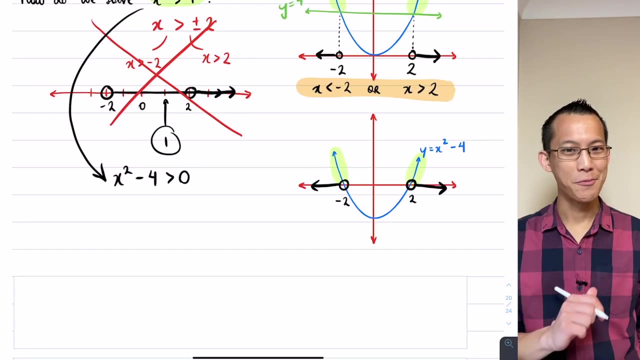 this way because I'm really good at finding where things cross the axis. these are intercepts. we've been finding these for years and years and years. so, mathematicians being famously lazy, if we've got a skill we've well developed, I want to hijack that and use it to solve these new questions. okay, okay now, as.